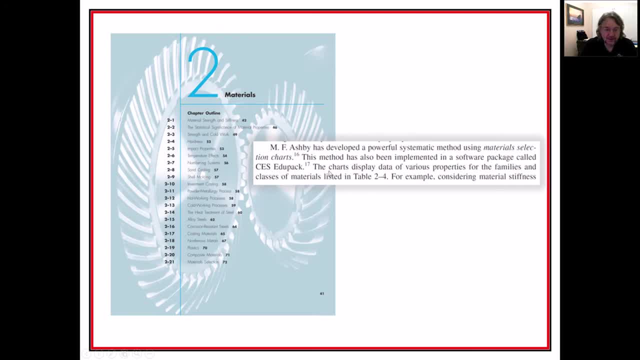 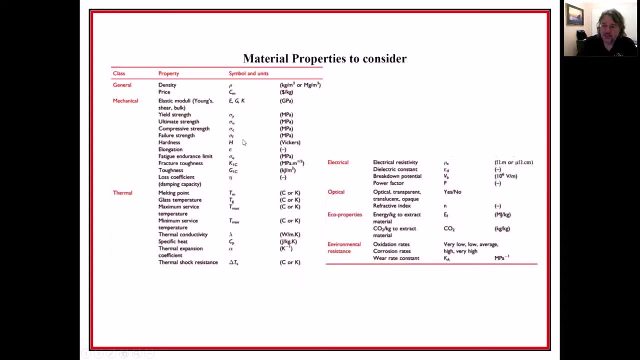 And so here's even alluding to the software that's available from them. So some material properties. There's lots of different material properties that might be important to us. A lot of times we just think about strength, or we might think, when it comes to deflection, Young's modulus, That's, these like related to the stiffness. We might also think about the density, But the cost, the price, is also something very important. We don't make it out of time, So we're going to go ahead and do that. 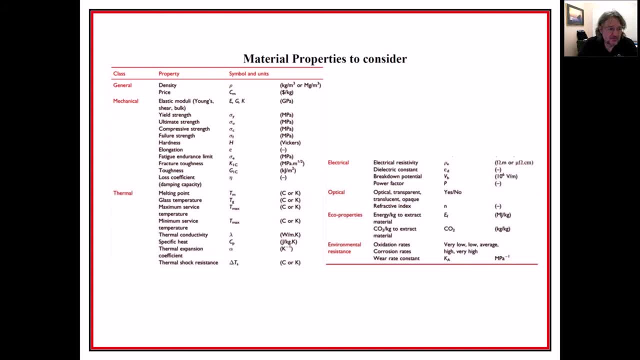 titanium. if it doesn't need to be made out of titanium, it's expensive. it might be strong and light and and stiff, but also expensive. so we have to, kind of like, come up with some priorities. there's a lot more to this decision. we might make a decision making matrices, kind of thing. 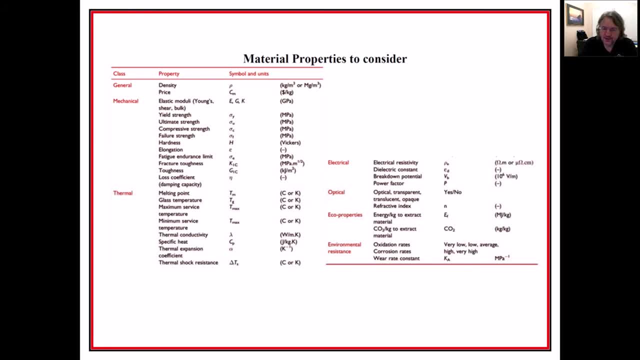 but for right now we're going to stick with just a couple really simple treatment of the thing. once again, this is a field of study where there's a lot really deep that we could go into. but also thermal properties might be something that we're going to look, we would look into. 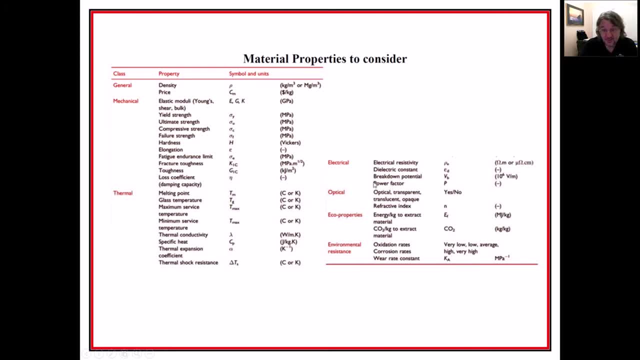 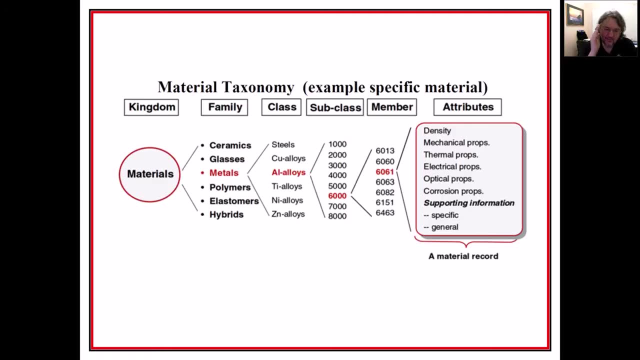 conductive, electrical conductivity might be something that we would want to consider, depending on the application. so, like there's, like you know, we could break down the family, the kingdom, the family, the class, the subclass, the member, and then like the attributes and so forth, so we could systematically break down. what kind of material are we talking about? 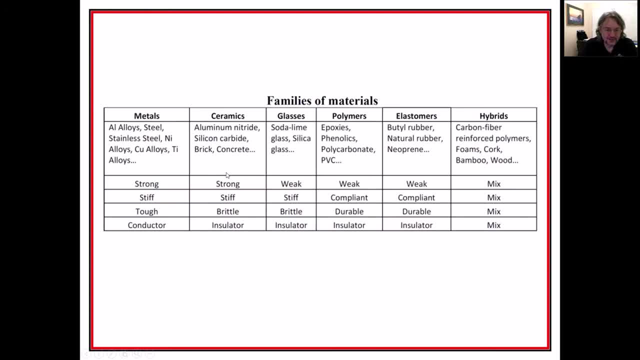 and in these like, for instance, uh, they all have from these different families right here- metals, ceramics, glasses, polymers, elastomers, hybrids- you could see that they have um a variety of like traits like strong, stiff, tough conductor, strong, stiff, brittle, uh, insulator. you know, comparing metals to ceramics and so forth, it's kind of interesting to try to think about those. 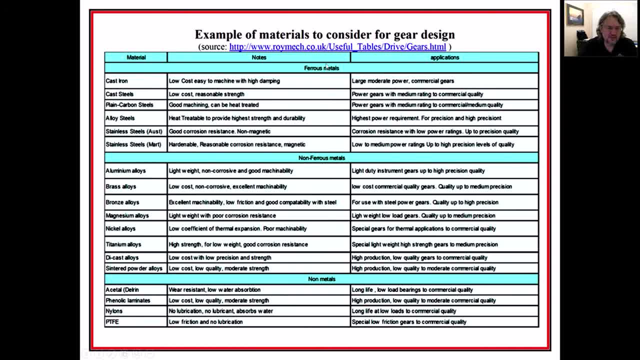 types of traits. this is just an example of something that i found from this guy, roy mech. you could look this up. he's got a lot of stuff. it's kind of interesting, some mechanical stuff. i have links to this on my useful links and resources, but here's some notes about different. 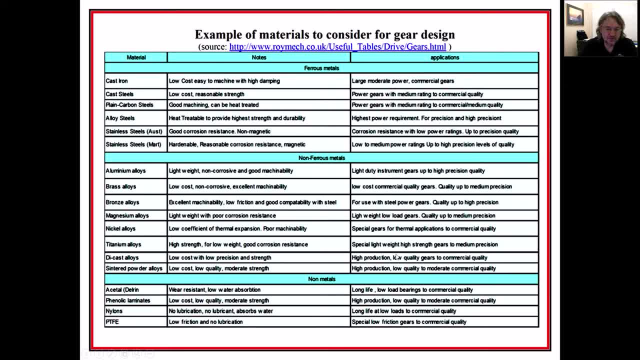 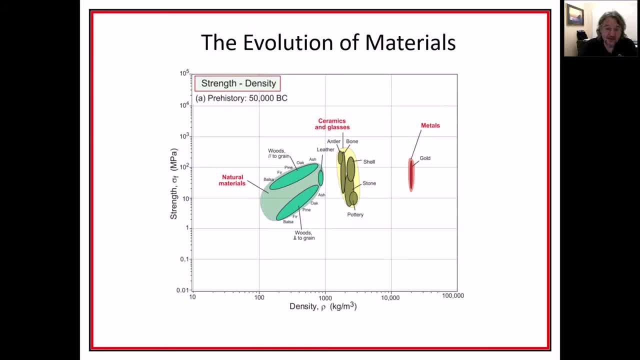 applications of various materials that you might want to consider right. so we might even think about, like, looking down on the applications process and going to the other side. these are some charts, that kind of talk about the history, and i find them to be interesting. maybe you will too. but we find the evolution, and this is prehistoric times. 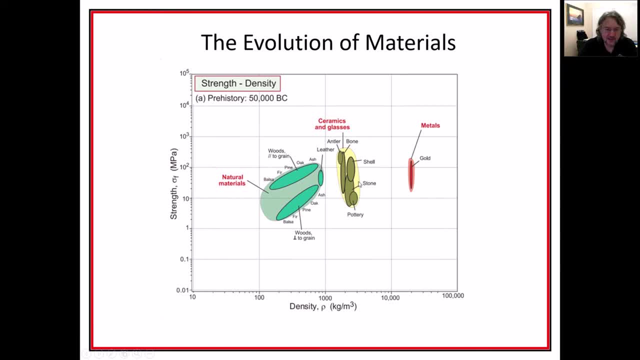 we had like we made- they made things out of wood, right, or they made stuff out of bone and shell and stone, and maybe they could find some gold and they were able to pound gold and and be able- maybe even be able- to smelt it a little bit and then 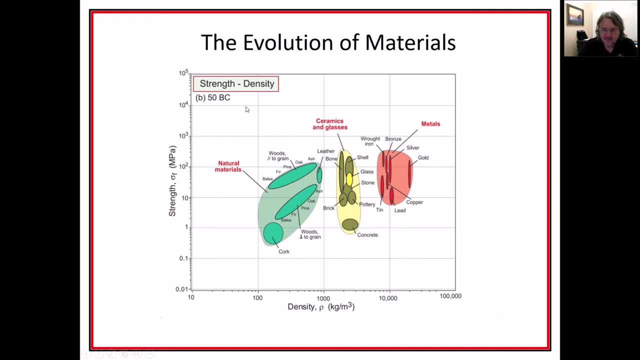 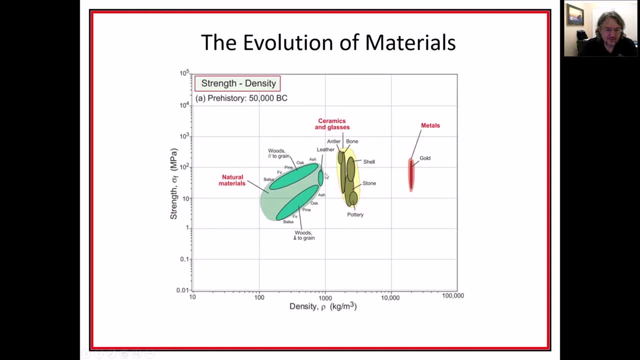 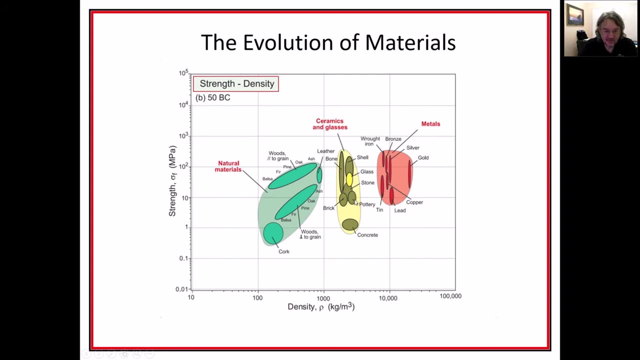 you know, in 50 bc- this is right around just a little before birth of christ- we had the natural materials- you know we might be adding cork to that, right, you know- and some some ceramics and glass. maybe where we actually can make some glass, we have pottery and brick and concrete where they. 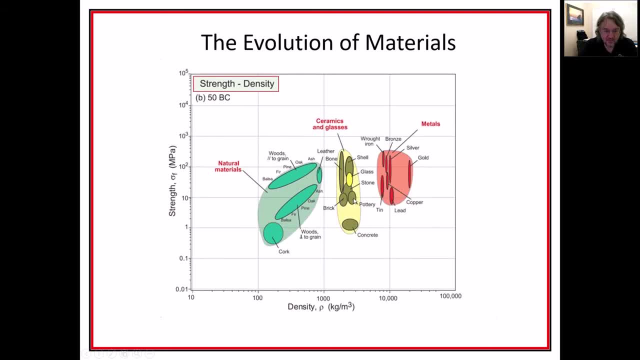 might have had concrete- it makes me pottery before, but now they're actually able to make something out of a type of concrete. i'm sure it's early concrete then, but You can see the metals have increased right from 50,000 BC to 50 BC. 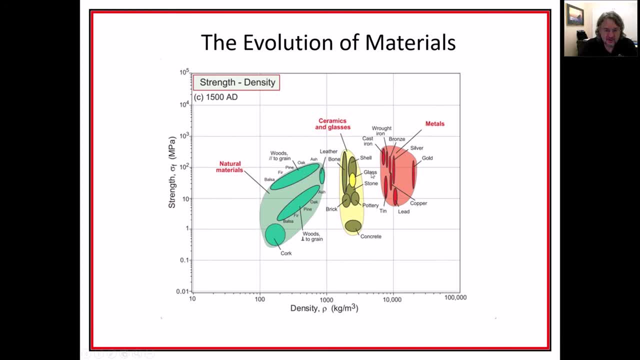 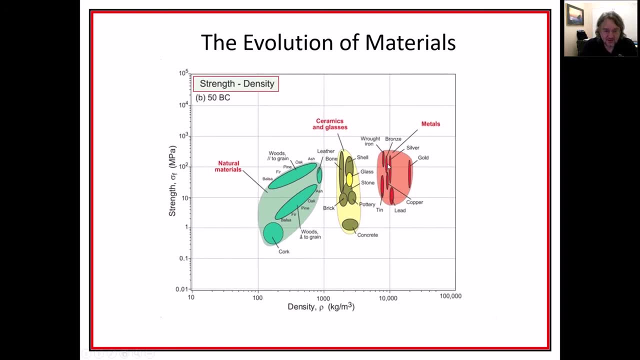 And then from like you, skipped forward to 1500 AD. you could see between here's 50 BC, you could see that there's more metals, like you know, not many more like this wrought iron. 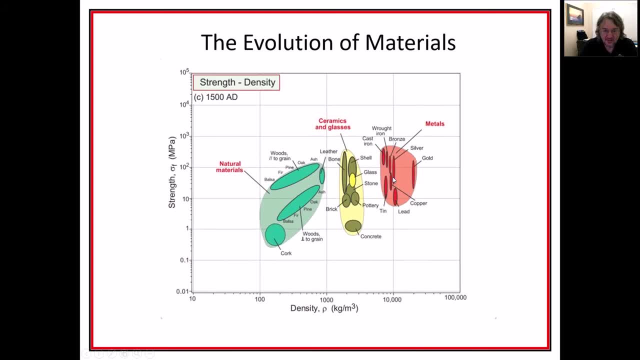 cast iron is part of that, not really terribly too much. Then we go to 1900, right, So there's 1500 AD. so, like you know, Columbus is just set sail, just found the new world. 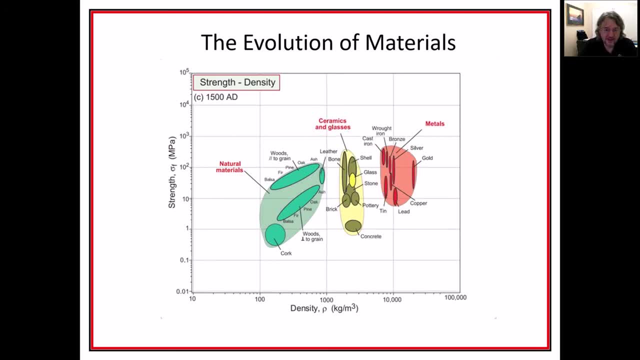 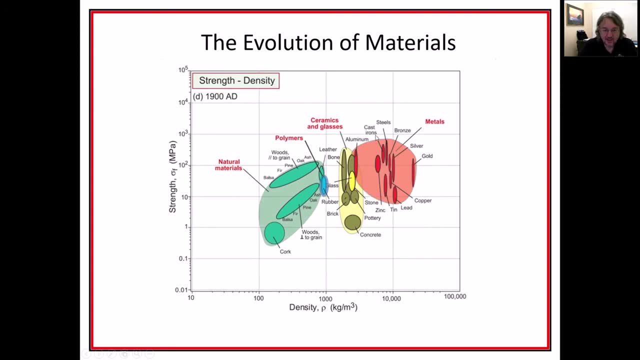 But now we get to like the beginning of the previous century And you can see that we have rubber now and polymers and some aluminum and some steels. That's good. We've added in some zinc, But I think aluminum is really nice. 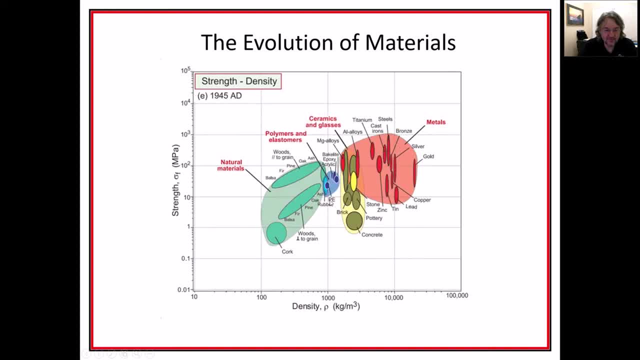 That's kind of the big progress that we've made in there and some of the polymers and rubber. But now we have like 1945, so like the end of World War II. You can kind of see we're jumping back and forth here. 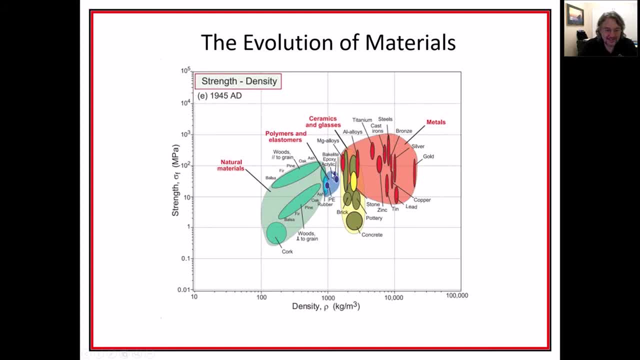 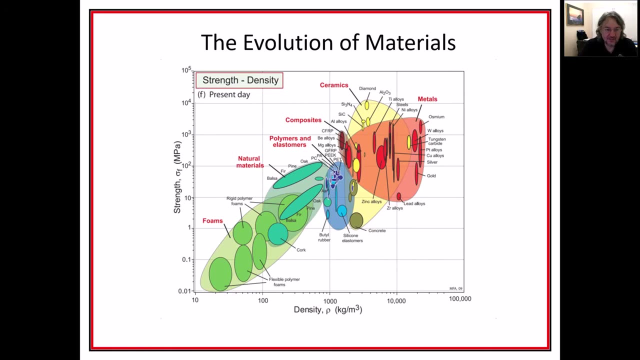 You can see the different types of. we have some more plastics that are going on And there's magnesium alloys and aluminum alloys and some titanium in there, right And then. but now we take a look at present day, right, So we have a lot of fun. 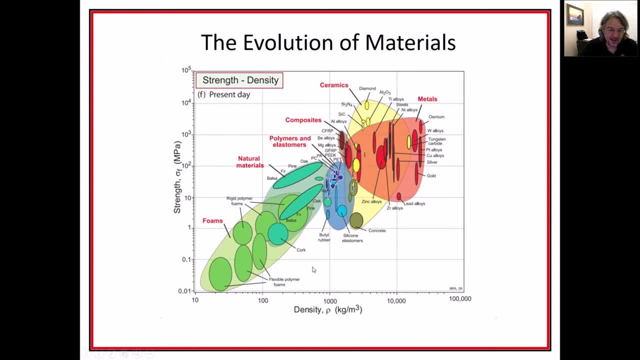 We have polymers and other polymers. We have some various other things down here in the polymers and elastomers. We have quite a few more ceramics that we're dealing with and they can be very high, And this is strength versus density right. 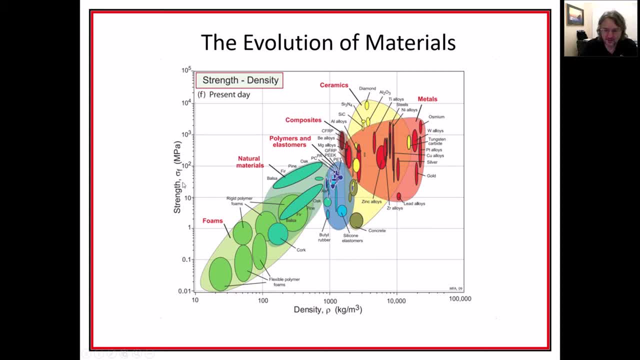 I should have said that right away, but you could read the thing and go back and look at it. These characterize we want something that's like lightweight and strong, And so, as we could kind of like, try to go up. 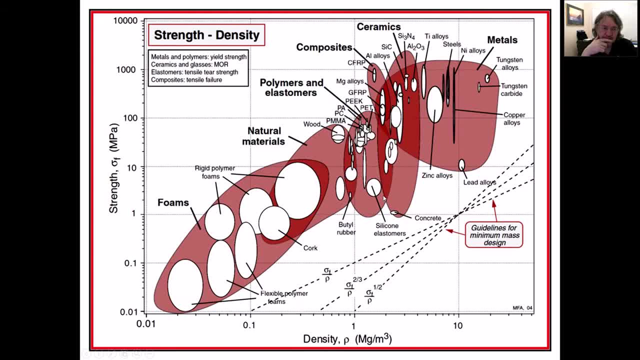 And so, as we could kind of like try to go up into this direction, So that's what these Ashby diagrams right Here's just strength and density, And we could see that they have these things called guidelines right here, And you could see that they have this kind of form that doesn't quite make sense. 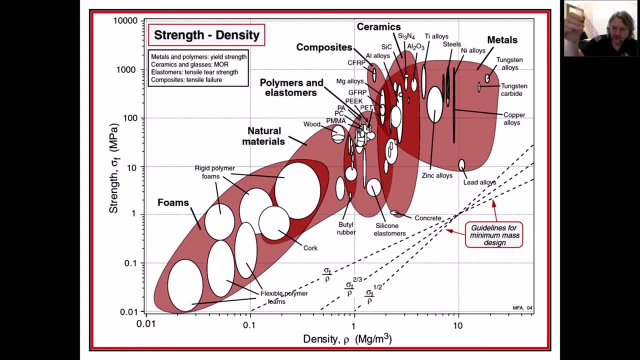 I mean, these are just like slopes where you might take a ruler. I guess the ruler would look better this way, right here, right? No, let's see that way. Yeah, okay, that way, Okay. Slide up and down through them. 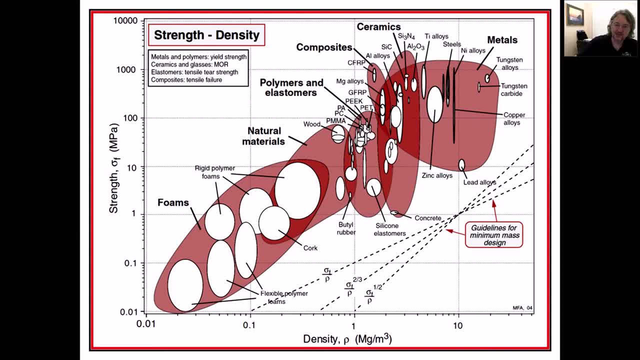 Let's see, going this way, My camera's backwards, isn't it? Okay, Anyway, so you could find for these guidelines, you could find like stuff that everything that's above it would be like acceptable for you. 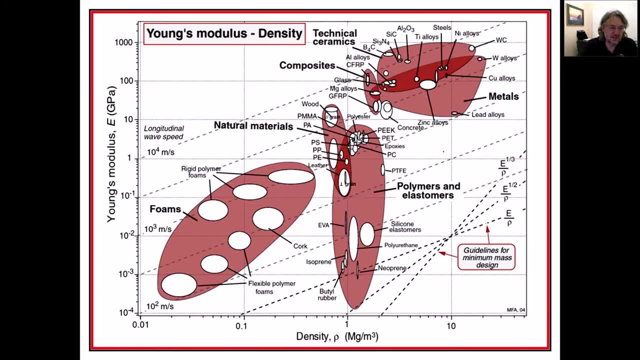 So you could kind of like narrow it down. But that's just strength and density. You could also plot out these traits for Young's modulus and density maybe. And you have D, So you could start looking for some of these different guidelines that we could run across. 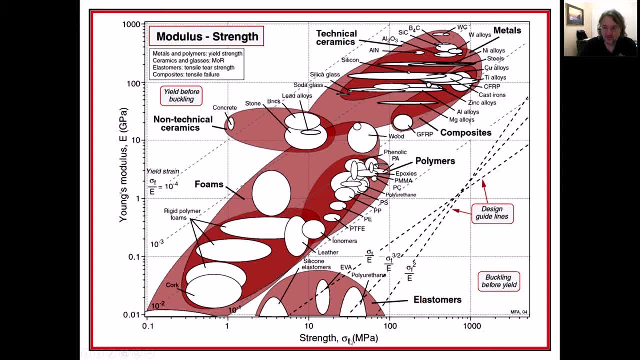 Or we might have Young's modulus versus strength, right? Okay, so we got density out of the picture, So you could start looking for some of these metals. you know that have high Young's modulus, So they're stiff but they're strong right over into the upper right area, right there. 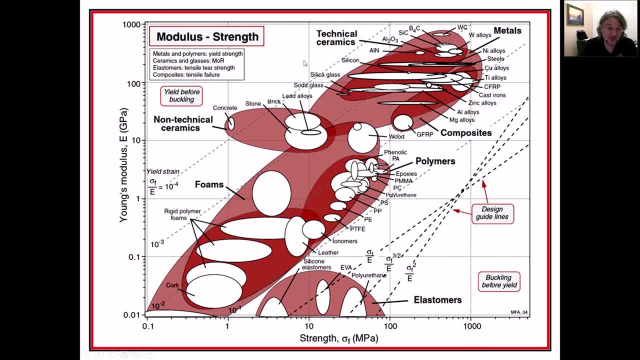 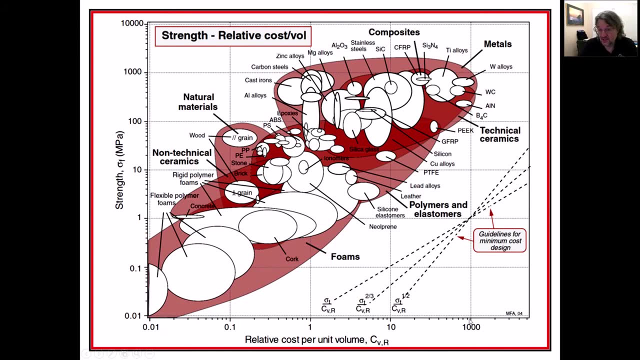 But maybe we want it to be strong but also flexible, right, So we might have like a low Young's modulus but a high strength right there. There's also strength versus relative cost. Now that's an important one to us, right. 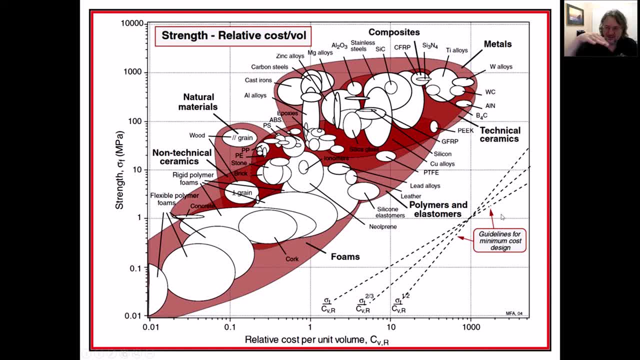 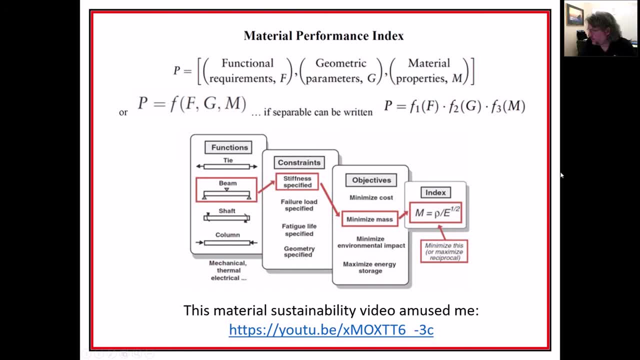 So we could kind of like take a look at these lines and draw those lines and then kind of sort of narrow down. So the method about which that we go to try to apply this is to create some kind of a structure, So it's a kind of performance index. 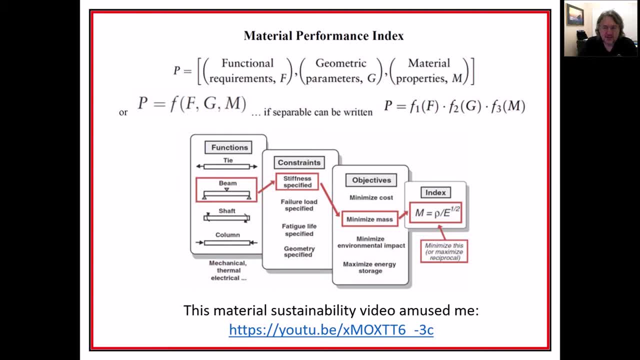 And we'll discuss how that's done by way of example. It's a little bit easier to see from example And you can kind of see that you know different things are a function of different parameters, So like we might take a beam configuration. 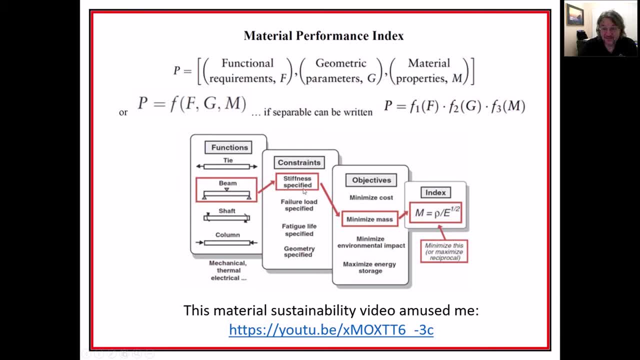 And we might say, okay, well, we've decided that the stiffness is specified And we want to have the minimum mass. So we put together, We put together an assembled equation right there And we see what it's a function of. 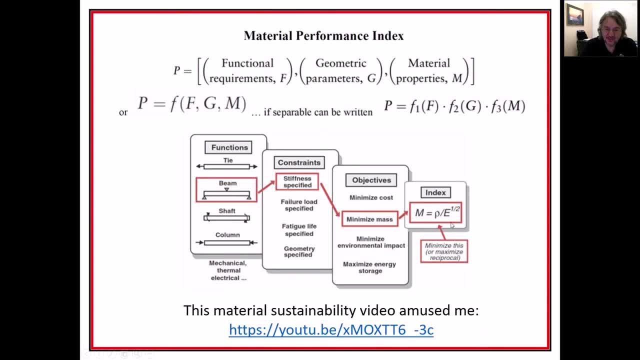 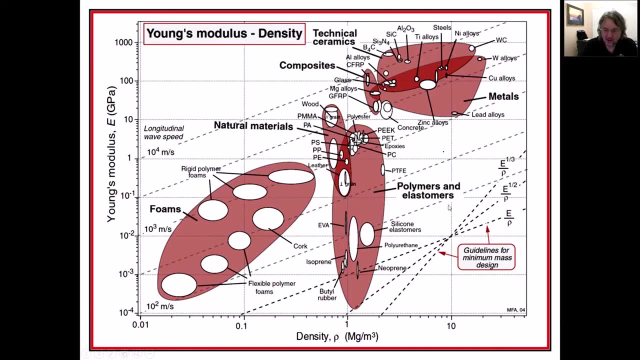 And then we use one of the lines right here So we can see that we have rho over e to the square root, right So where is that? Okay, so now this is reciprocal right here. right, So e to the square root, right here. 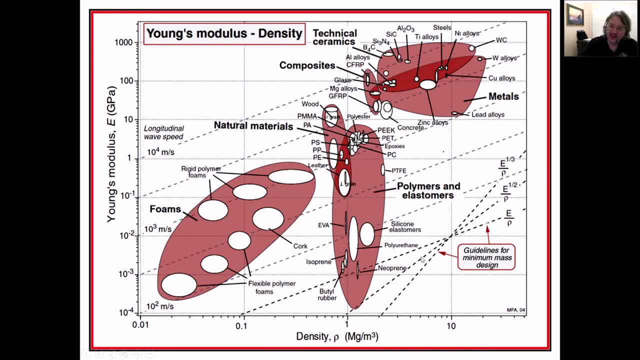 So here would be the line that you would use to try to say: okay, everything above this is going To be something that's going to be a material or anything that's on that line. right, there is like maybe we could is alternate materials that we might want to use. 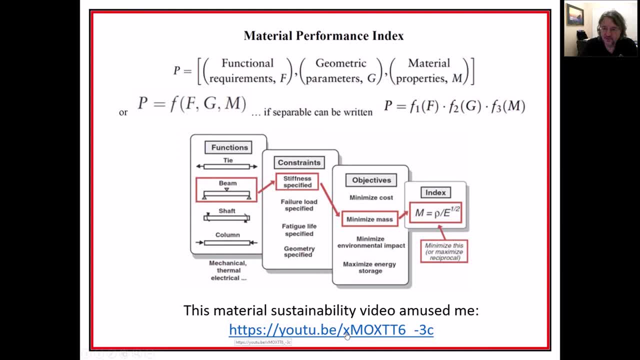 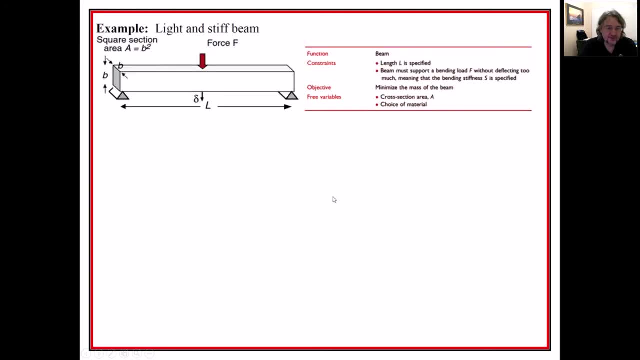 That's the big idea. There's a YouTube video here. You could click on this. It's kind of funny, but it's not going to take up our time. So here's the basics of this area of two examples, And I will go through them. 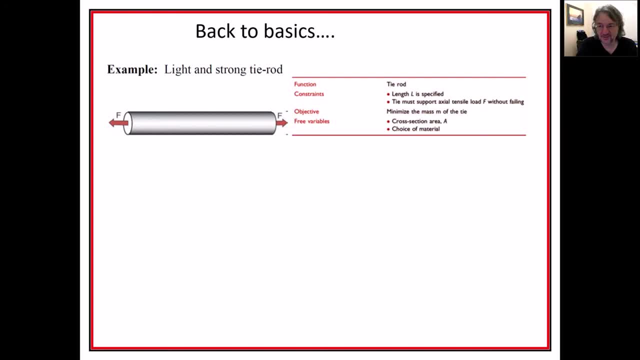 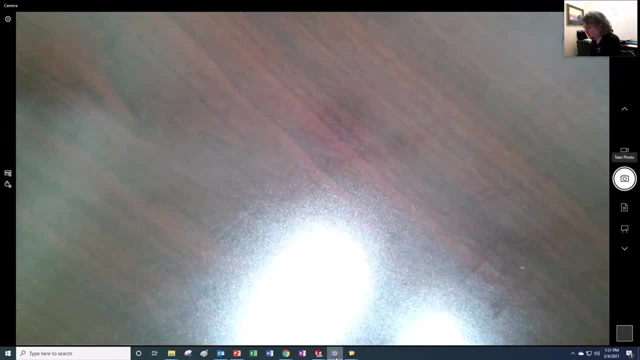 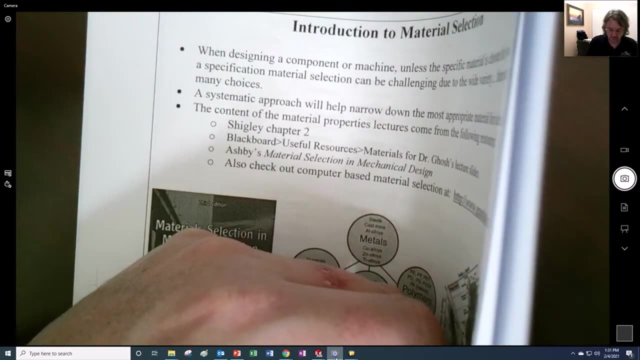 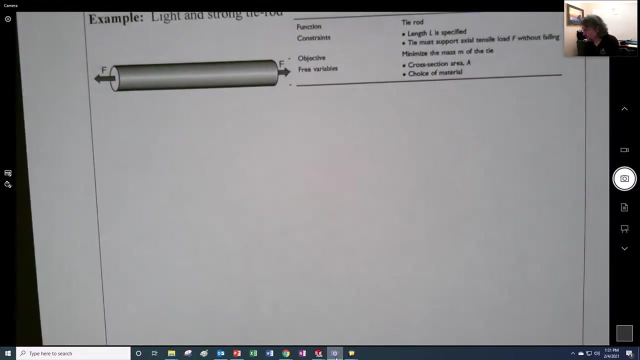 I don't know if we'll be able to do this in class. It's kind of ambitious amount of stuff for this class. So let me see here, And I have this all written down, Okay. so here we have that first example right in there. 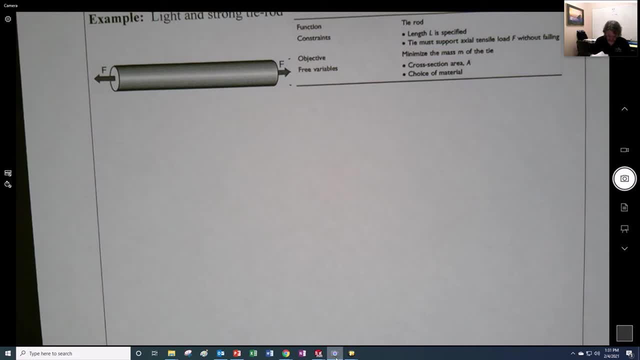 So I'm going to go ahead and write this down for my performance index. This is not that one. We'll just fast forward all the way through this one here. Okay, Okay. So Let's see, Let's see, Let's see. 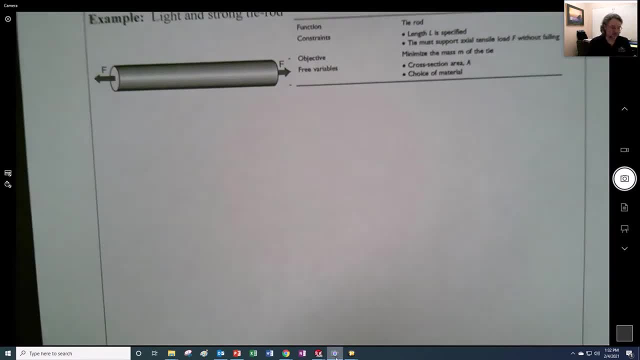 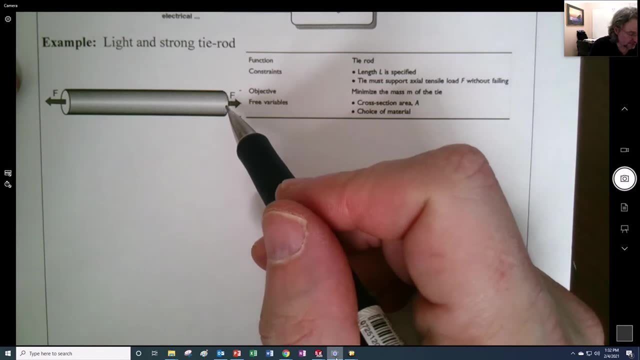 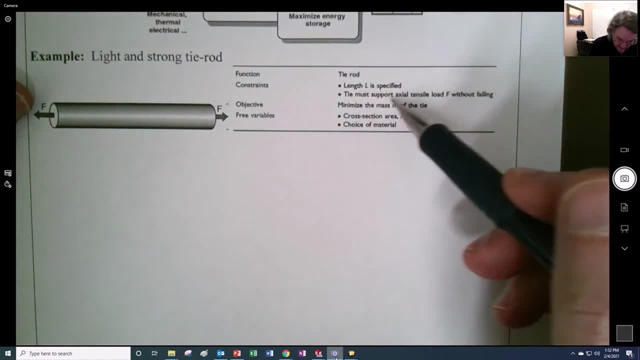 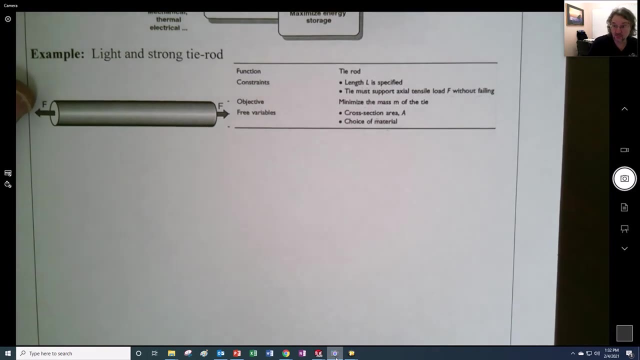 And the length is specified, and it must support axial intention without failing. And our objective is to minimize the mass of the tie, and the free variables are the cross section and the choice of materials Right, So we can… available to us as a designer to make choices. so, first off, we figure out what 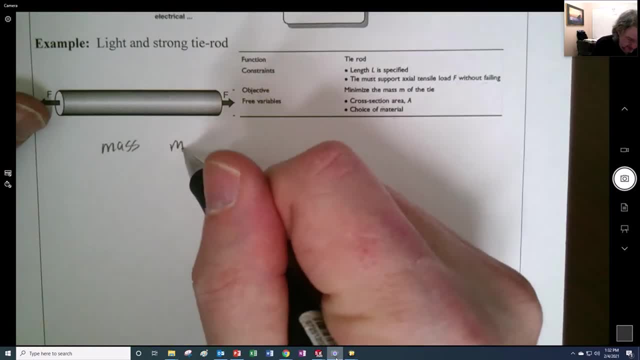 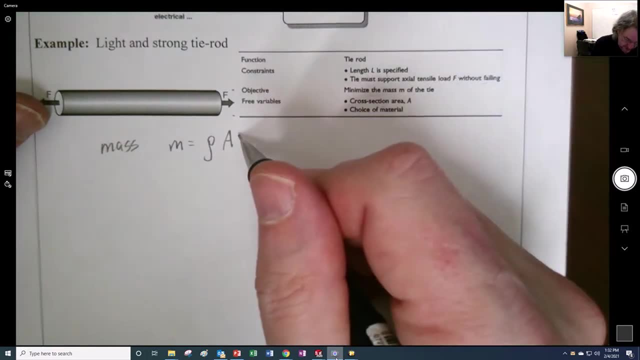 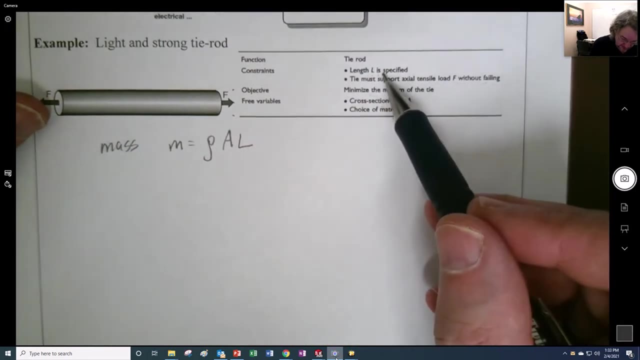 the mass is. well, the mass could be. we could find that if we know the density and we have the area right, you'll notice that that's one of our free choices. times the length right here, right. so here's the length where the, the length is something is specified, area is something that we are free to choose and 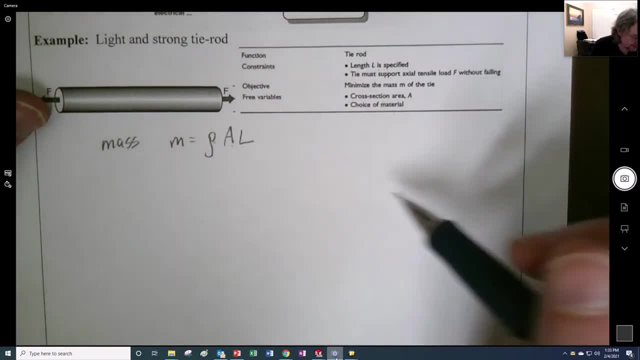 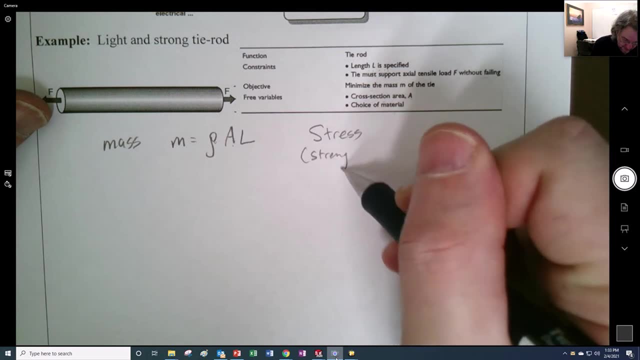 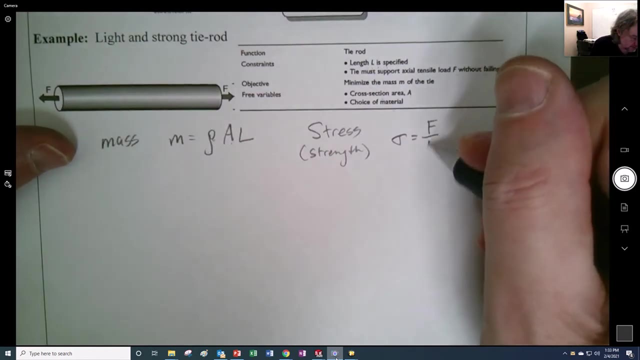 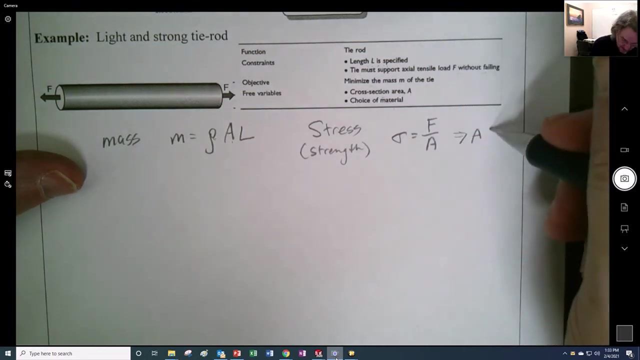 row is something also as part of our material right there. right, we can also say that stress, which is related to strength of the thing right is going to be, Sigma is equal to F over a right. so what we could say from this is we could write this thing out and say that a was equal to F over stress. right there. 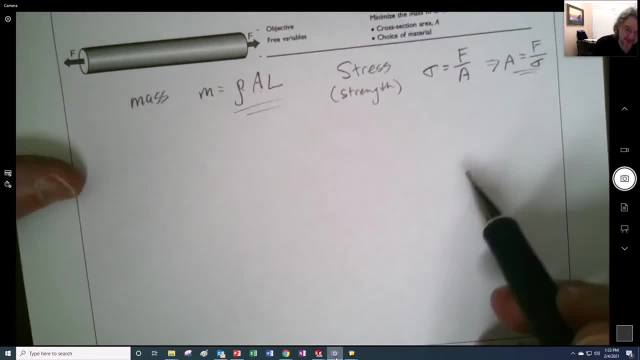 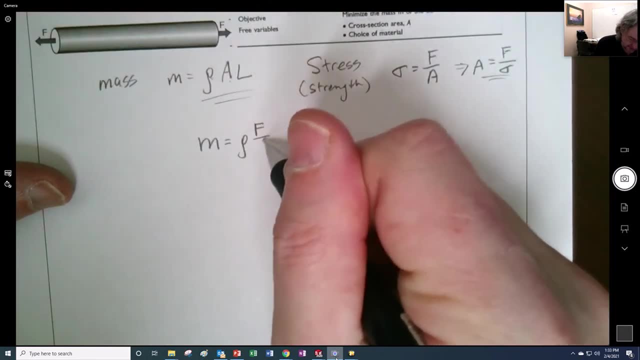 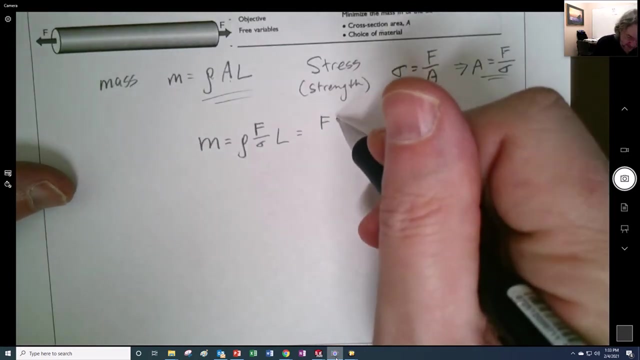 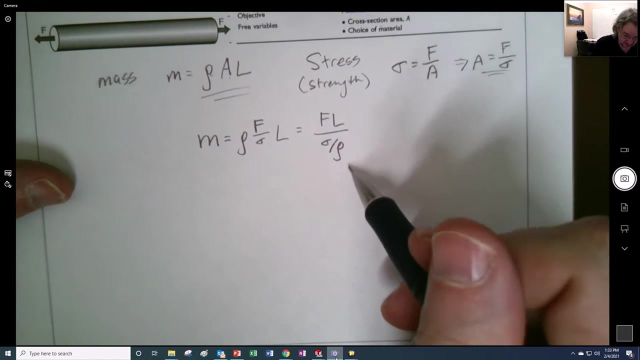 and we could combine these two things together and say that the mass was going to be equal to density times F over stress times L, and what we'd say. we could rewrite this over here. we say: FL is divided by stress, divided by row. right here, now, this thing together, right here, is a. 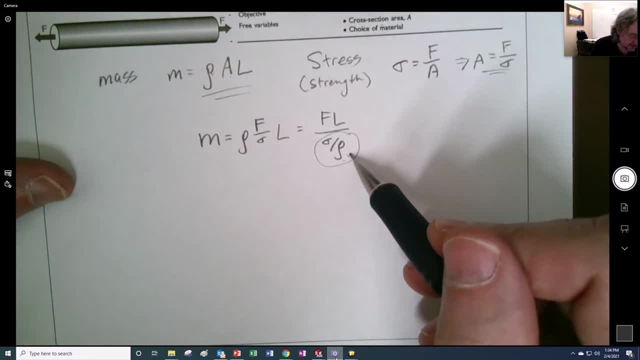 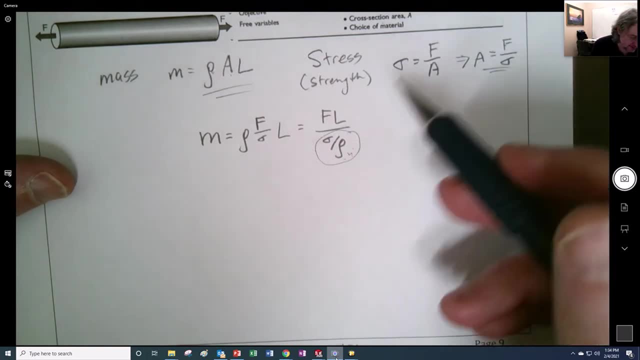 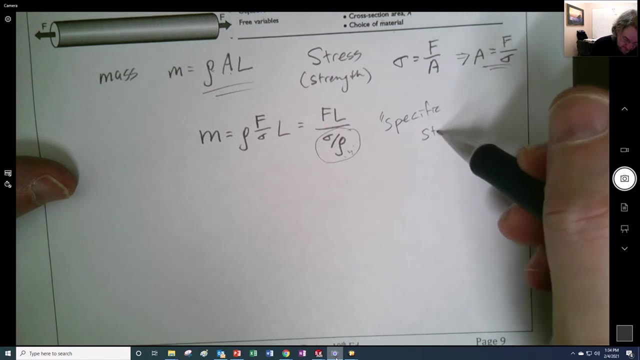 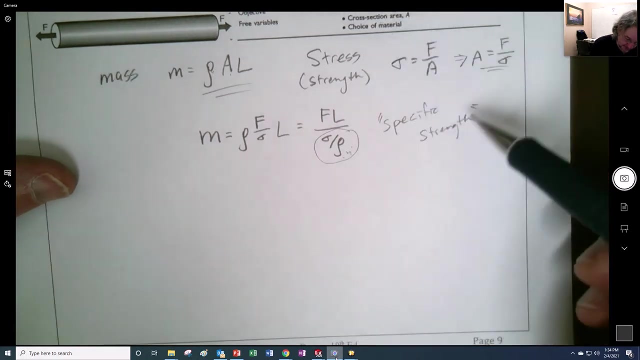 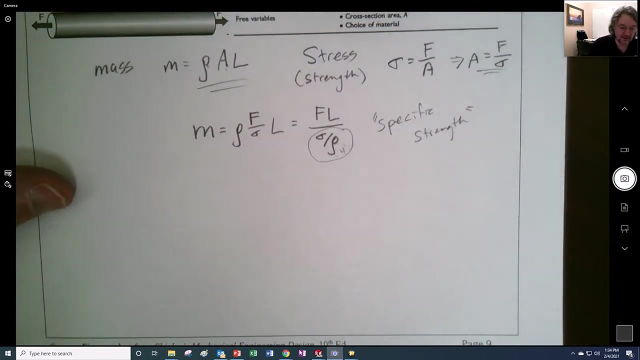 performance dependent index right here. right, so we could take something and we have a- we could call this, if we wanted to- specific strength, and our objective is to minimize the mass of this right. so we would use this um line right here. let's see, let's go back to these, to these lines, and do we have? 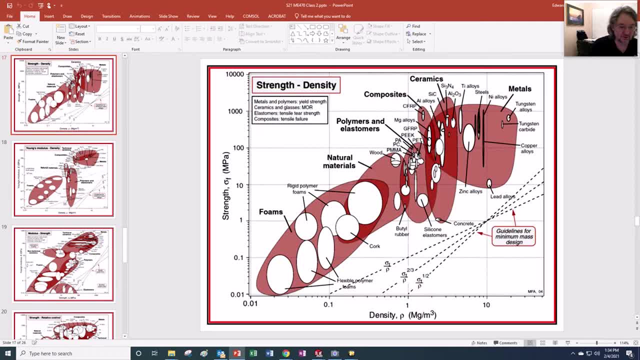 one that looks like this: right here, boom. so right here you see that stress and that density. we would use this line right there. these are the guidelines for the minimum design that we would place onto this right here, hypothetically. now coming back into our problem here, what if, instead? 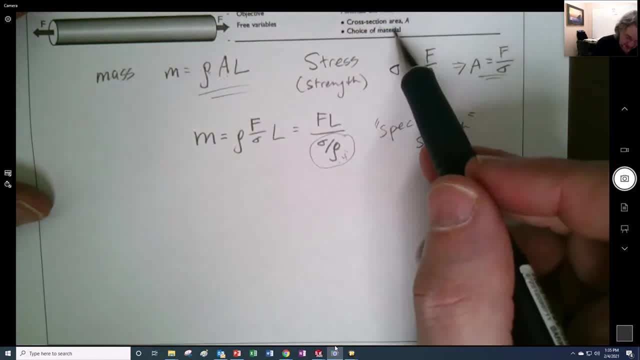 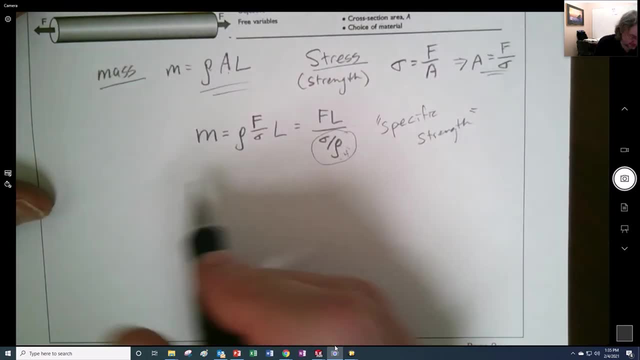 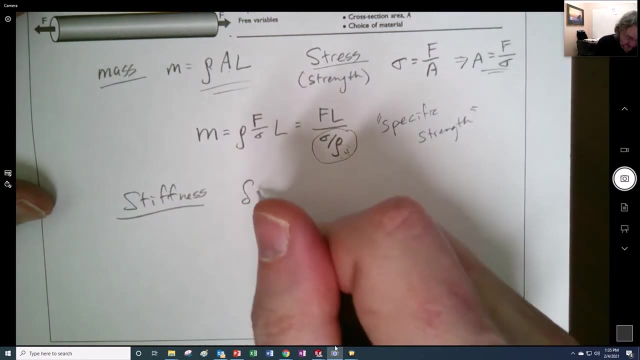 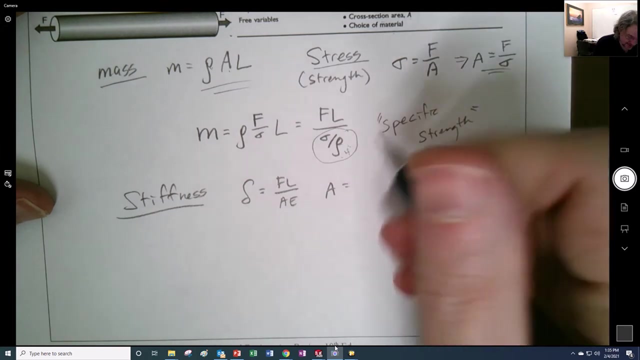 we were going to say that we were going to do some amount of the stiffness was also something that we would care about right here. so there's here's a relationship right here, here's a stiffness relationship, and that's going to be for rod, FL displacement, FL over AE, so we can say that a was equal to FL over. 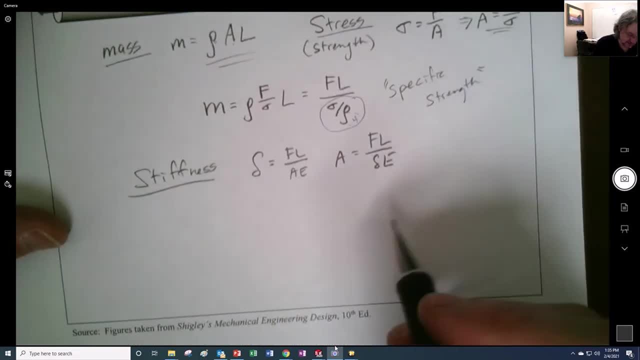 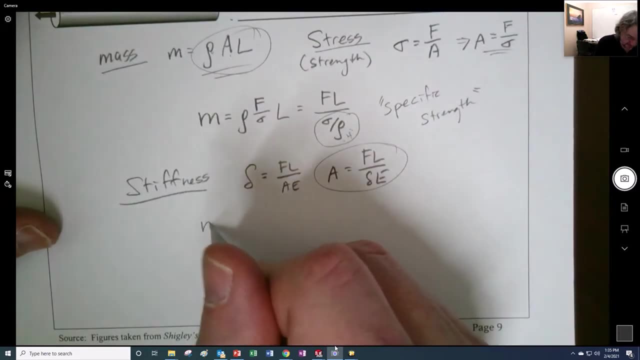 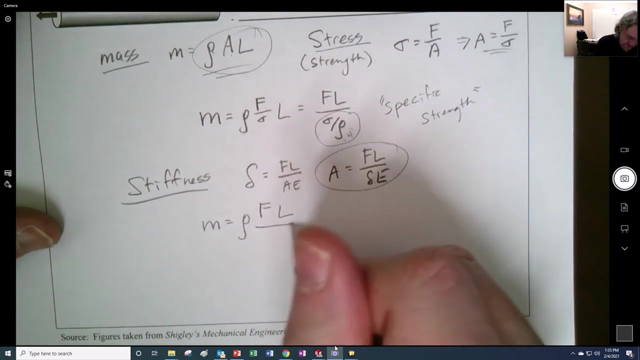 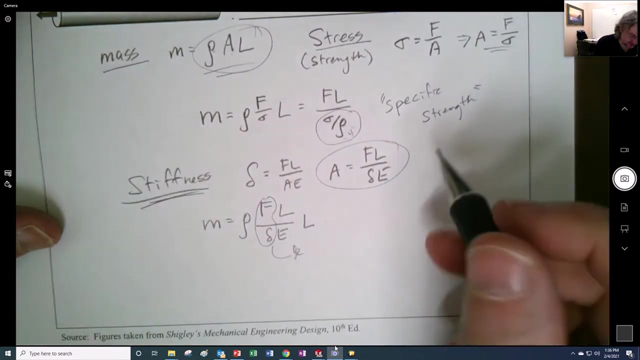 del E, and so if we were to place that back up into here, we could now say that the mass was equal to density. FL del e times L. notably that, right there, F over del is a is stiffness. right there, right there, right. so there's our, there's our stiffness. 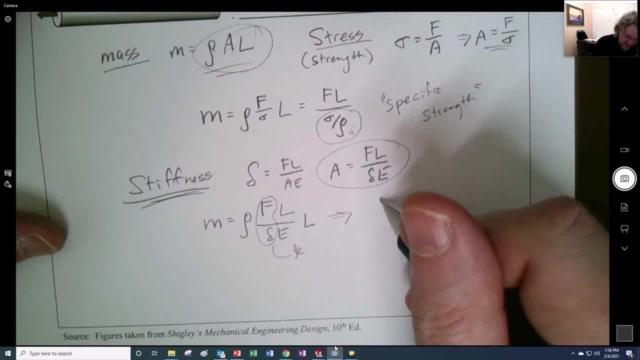 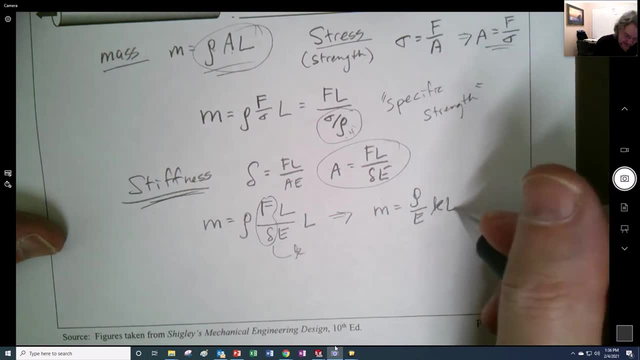 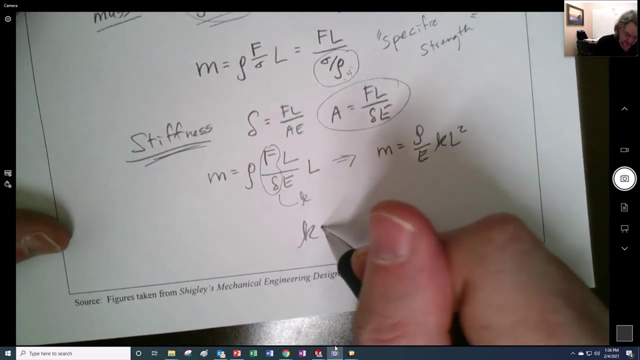 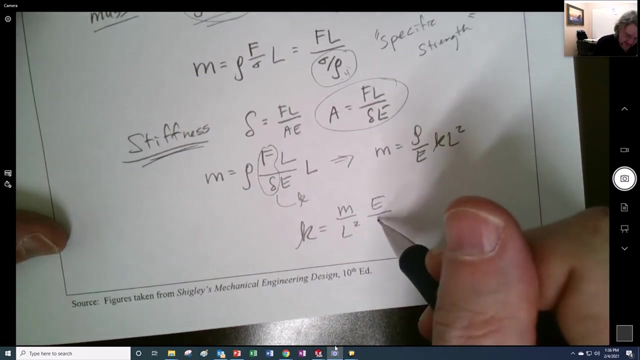 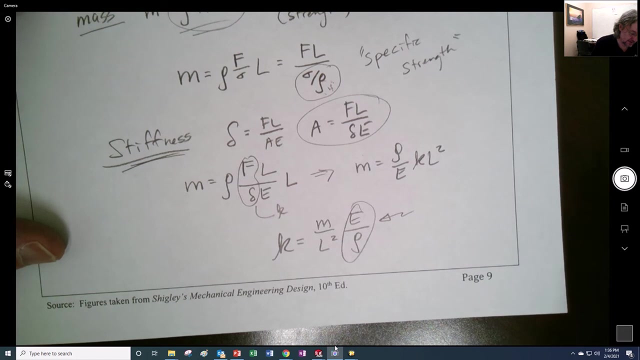 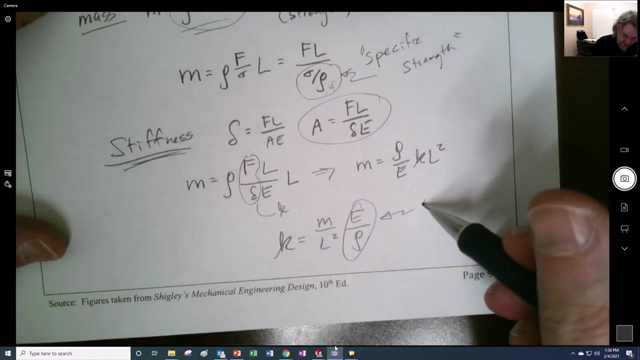 we could say that what we have here is m is equal to del e k l squared right here, or maybe stiffness, writing the whole thing out is m over l squared e del. so right, there is a performance index right here. so here's one performance index, here's another that we might call specific. 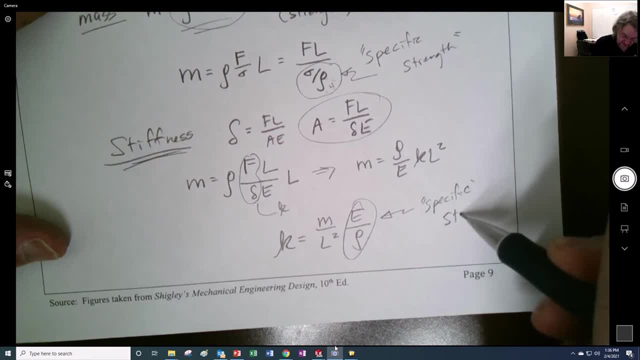 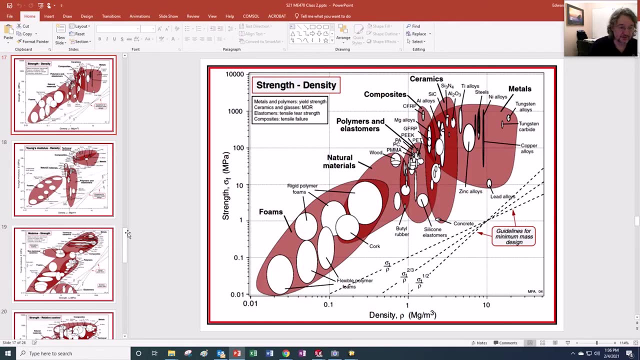 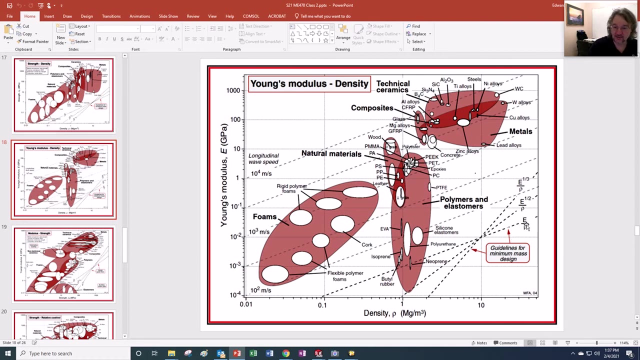 stiffness and we would use instead um. and we would use instead um this right here, right, so we were taking this line right there. e row is our specific stiffness. that would we use as our design guideline and we would take that and translate it up and down to try to find lines, and you can even see. 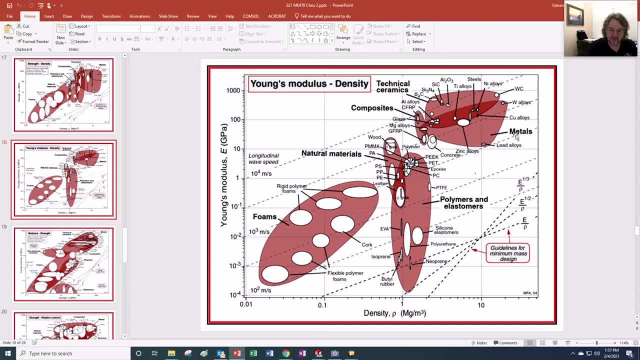 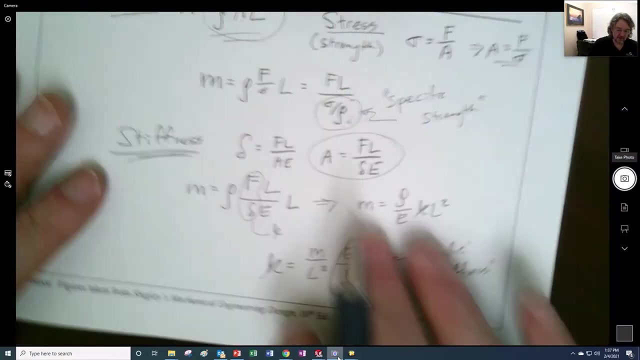 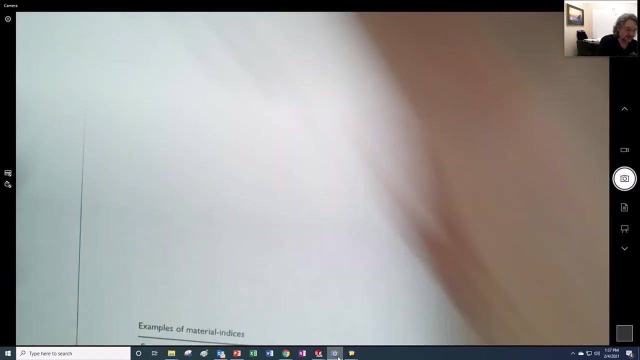 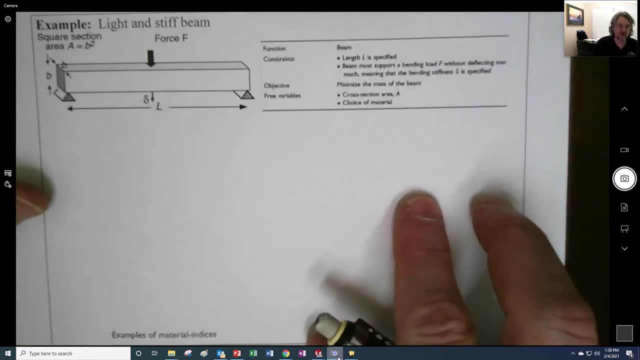 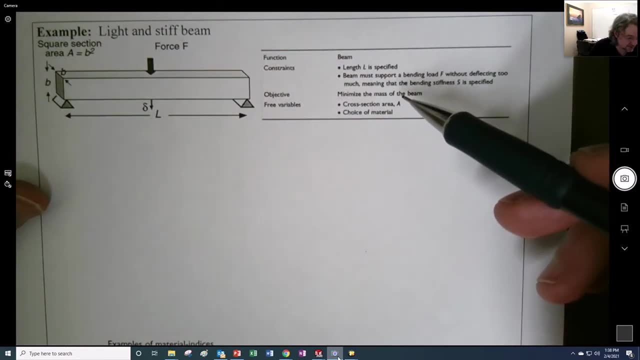 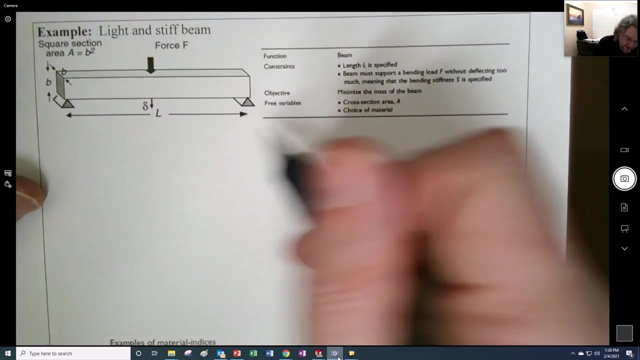 to it so you had some familiarity with it somewhere in your career. if you now, if we want to have light and stiff and it's beam bending now, so you can kind of see a little bit of a comparison to the thing, we know that the the the length is. 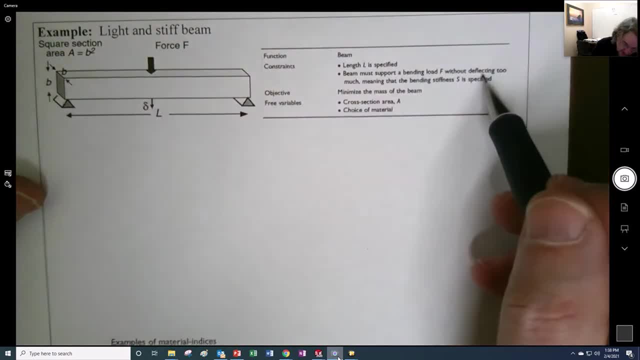 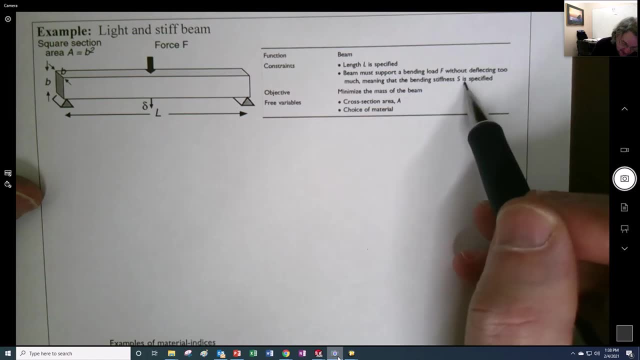 specified, the beam must support a bending load F without the, without deflecting too much, meaning that the bending stiffness is Stefan, specified right, or that might be Dell. I think that maybe this s, I think it would be K, maybe I would have called it so we can. the cross-section is what we're going to. 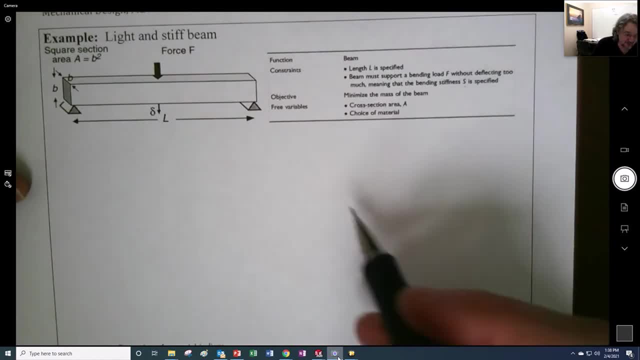 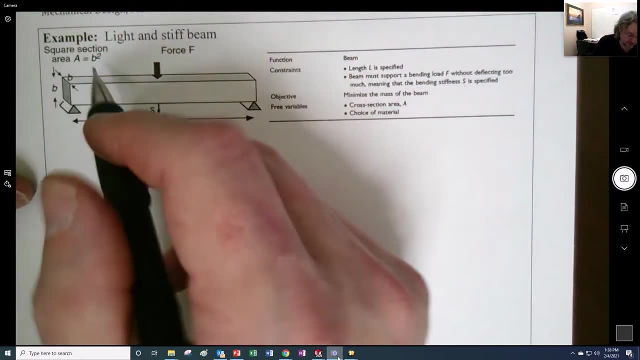 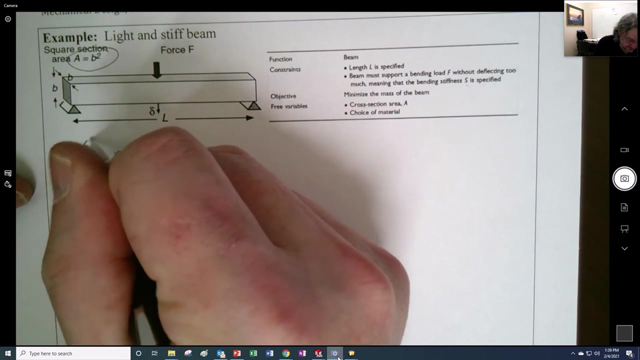 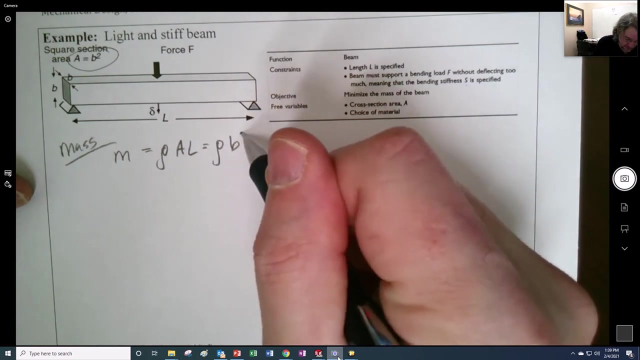 choose in the choice of material is what our free choices are going to be so, and it's got a square cross-section that really helps us this. the area is a B squared, so the mass of the thing is going to be equal to row a, L, and therefore B squared, L right and the 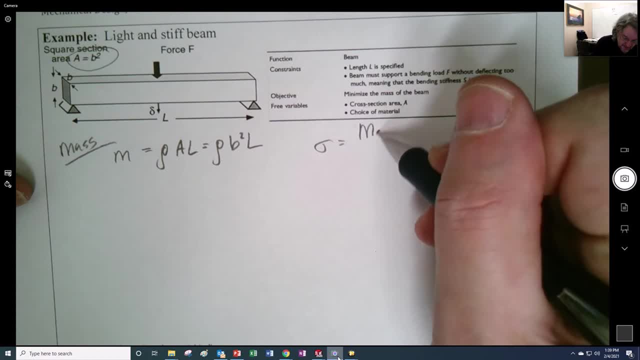 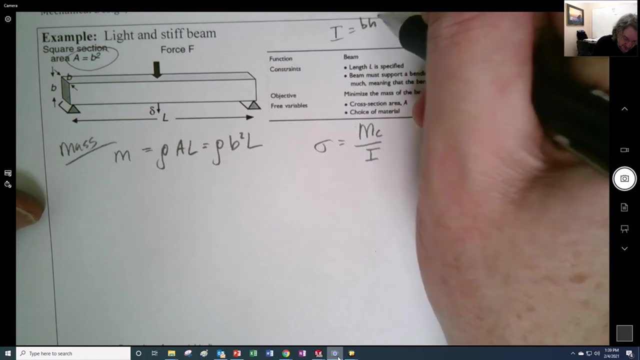 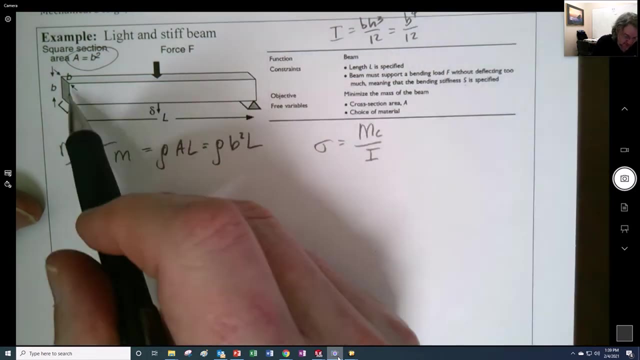 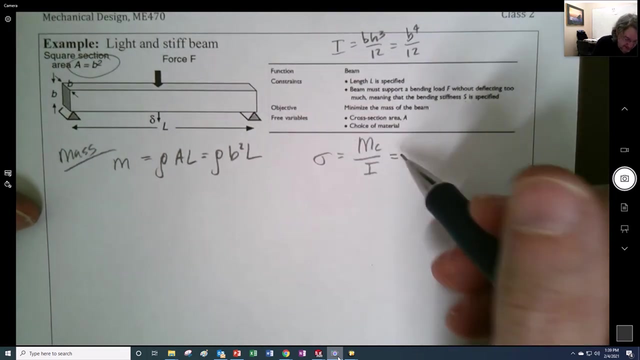 stress of this is MC over I, but we know that the cross-section of this is b H cubed over 12, which for us is actually going to be B, fourth over 12, right, because it's B by B. on to the thing, and if we go ahead and do a free, 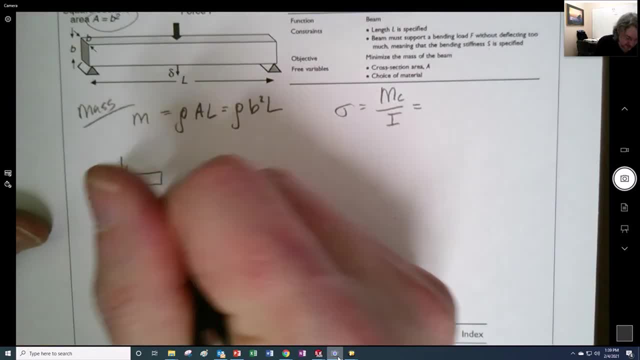 body diagram and reactions. here's our F. we know that the reactions are going to be F over 2 and I'm just asking this to determine the score will be like. half is the equation, and if we look at the �든 on the right side of the diagonal�, well, this was a normal reaction. stack on the. other side of the diagonal. so we're going to use something that was kills up more. and if we don't have it, then what happens if this Yang speaker is all going to go all the other right, so exercise. so, unlike starting X, should've we say: this is the angle here where all 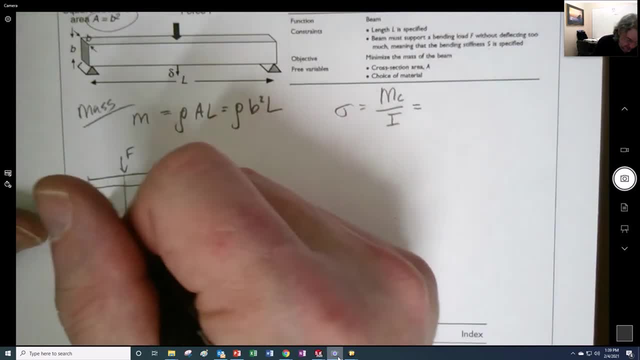 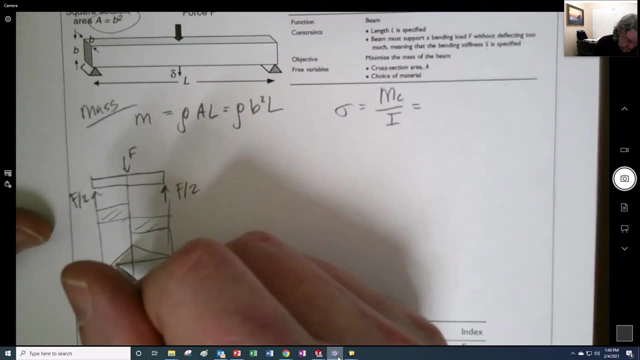 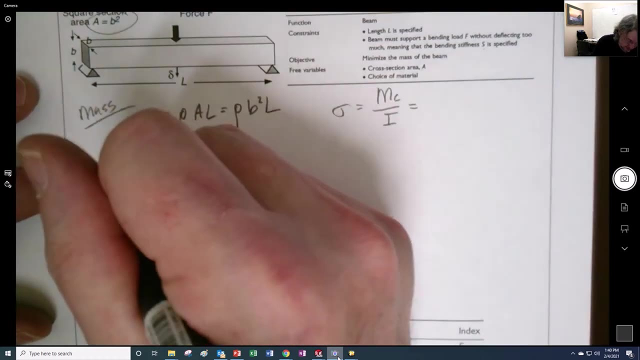 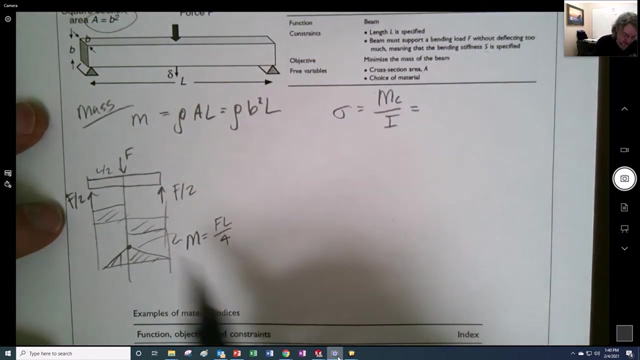 And F over 2, and the shear moment diagram. we get this right here. We would get that maximum moment right. there was going to be equal to, because this is L over 2, so that was going to be actually F, L over 4, right. 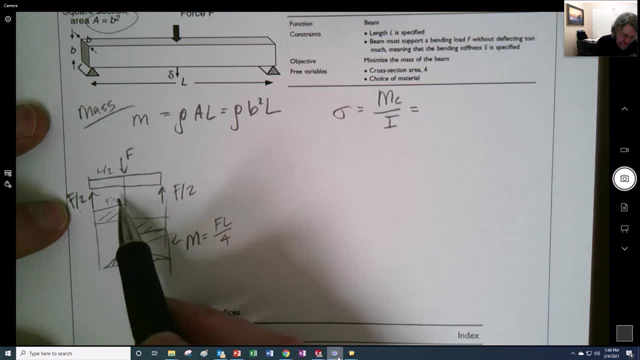 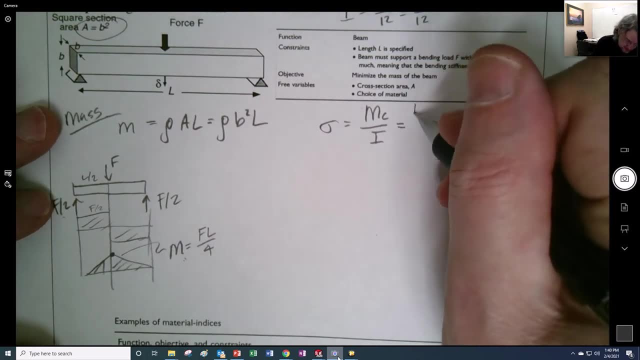 So it's F over 2 is right here: F over 2 times L over 2, so that's the maximum moment. So we would put this in here and go F, L over 4,, B over 2, and then B 4 over 12.. 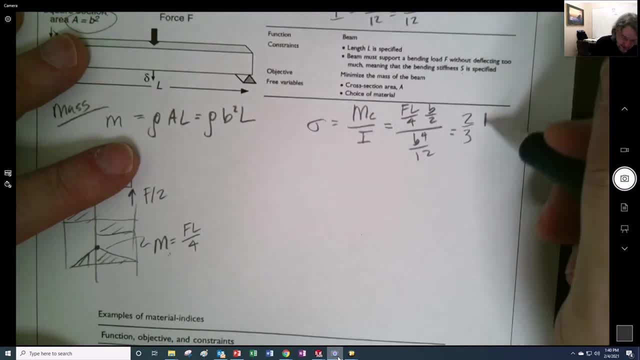 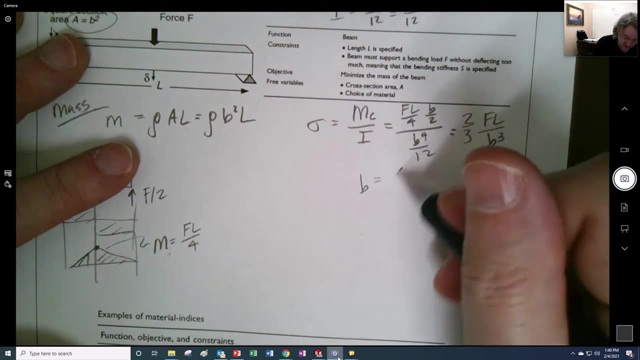 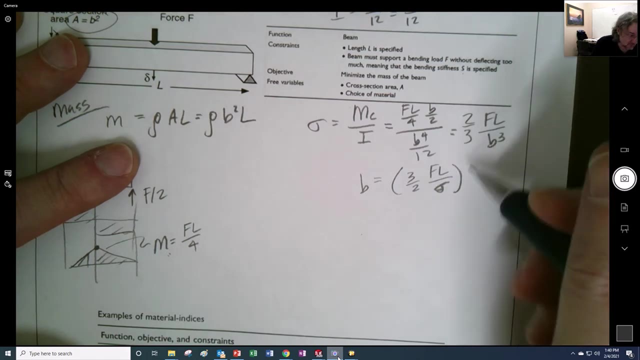 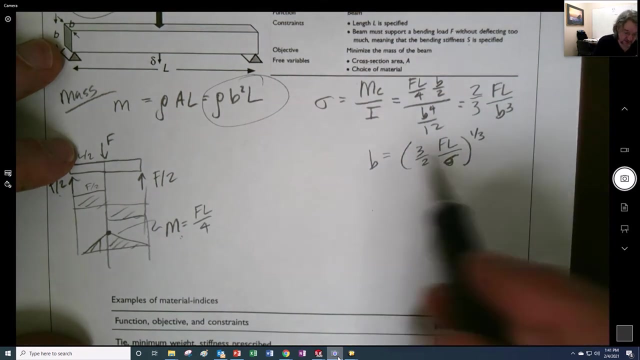 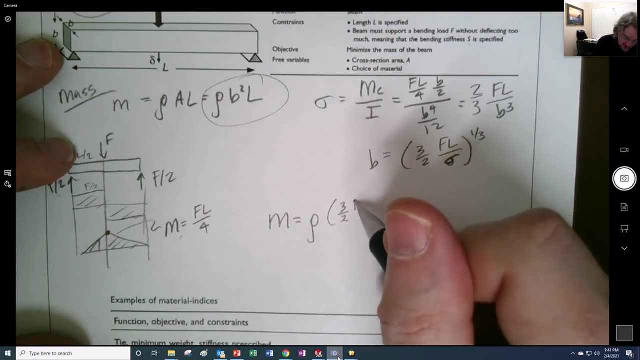 And what we find? we get 2 thirds F L B cubed so that B was equal to 3 halves F L, stress to the 1 third. So we could place that back up into here and write out that the mass is density: 3 halves F L over pi. 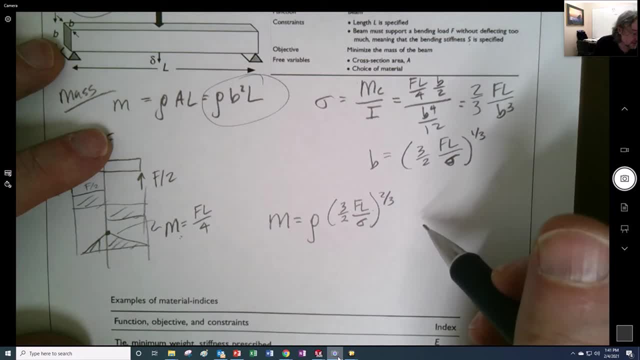 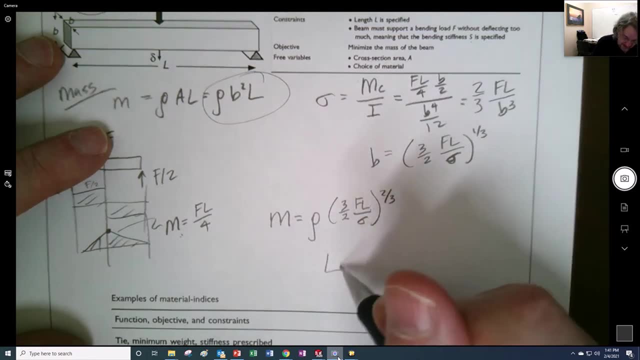 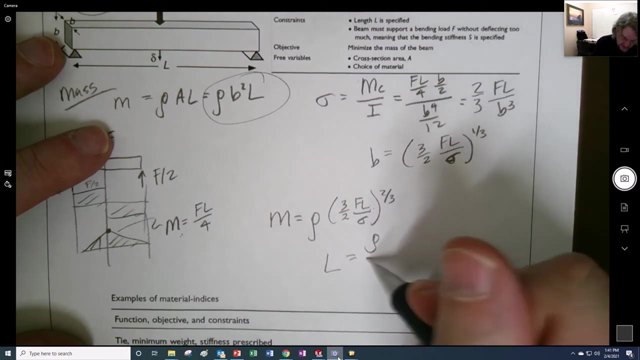 2 thirds. right there, right. So now, if we're going to try to figure out if the length is, if the mass is something that is set right here, we could bring that back out and say that we have density divided by strength, 2 thirds.